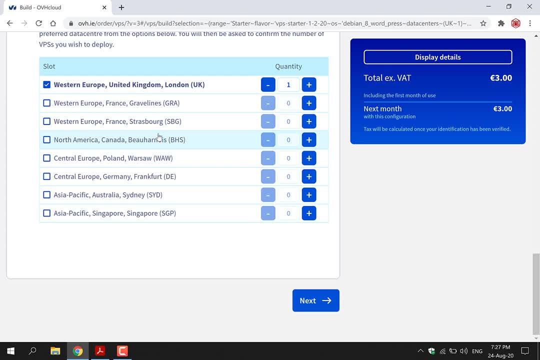 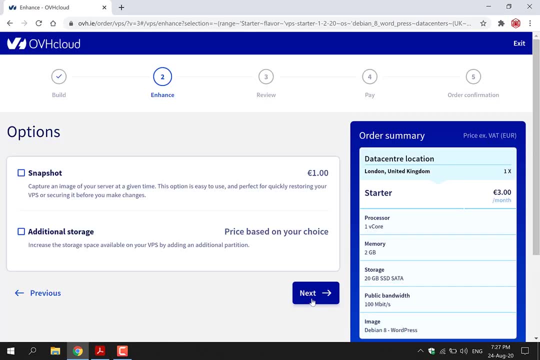 location. The best server for you is dependent on your IP address. As you can see, the UK London has been pre-selected for me and I'm going to stick with it. Click Next and click Next again. You'll now be brought to the order summary page. 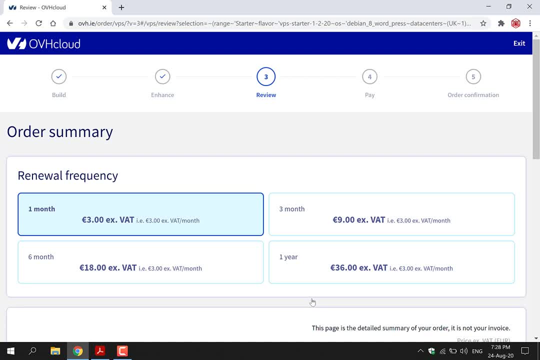 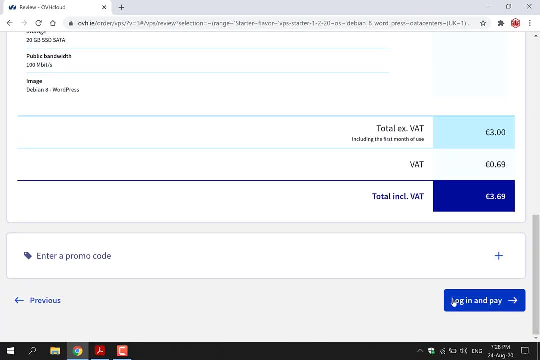 where, as you can see, it's 3 euro excluding tax. That's about $3.50, which is really cheap for a virtual private server. Scroll down and then click login and pay. If you don't have an OVH cloud account, you'll need to register and create an. 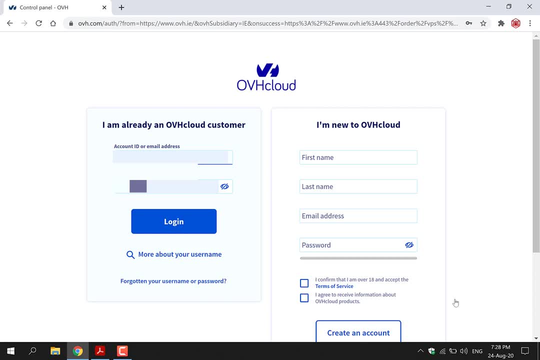 account. If you do, then you simply click login. You'll then be taken to the billing page where you'll need to put in your address and your billing details to make the purchase of the VPS. I already have a VPS for this guide, so I will not. 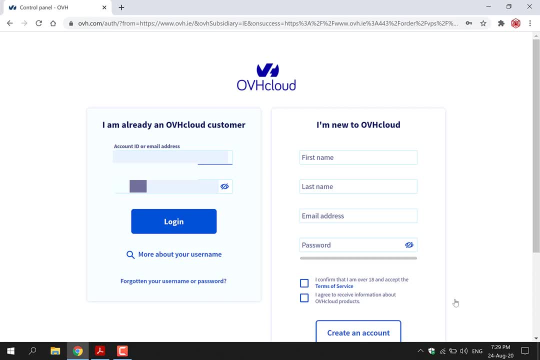 be buying another one. Once you've purchased your desired virtual private server, you'll be emailed the details to your VPS. You will not actually need to log into the control panel of OVH, as the login details provided in the email will suffice. You can, however, log into OVH's dashboard to do a server reboot or to 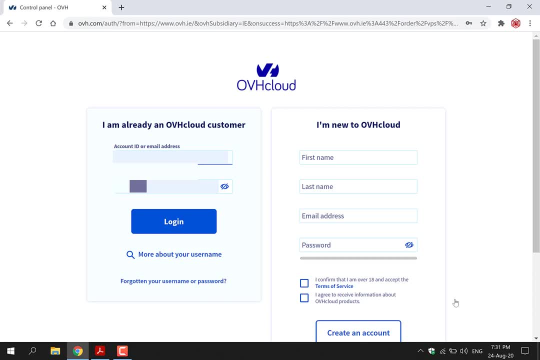 reinstall another operating system or an image. Okay, great. so once OVH has installed WordPress, you will have all the login details emailed to you. I have already downloaded the login details from my email address, just for privacy sake, so I don't need to go back into my emails here, So I'm just going to open up. 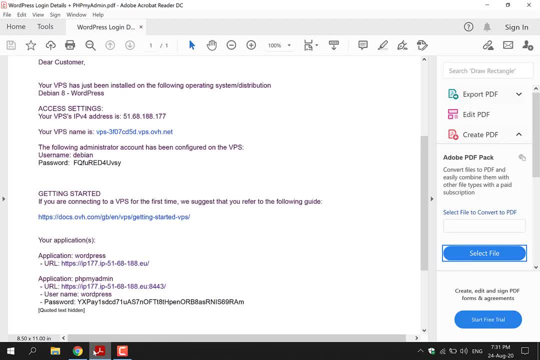 the PDF that contains all the details to log into the WordPress site. So, as you can see, the email contains the IP address of your server, the name of your server, the VPS on OVH cloud, the SSH login details and then what's really. 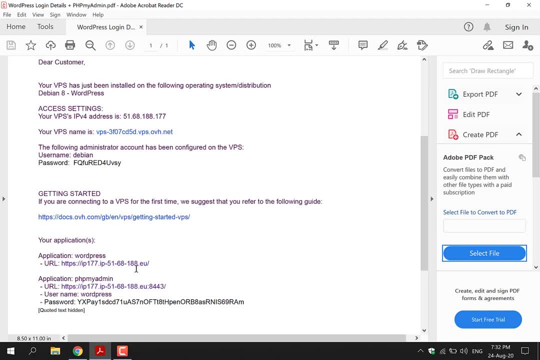 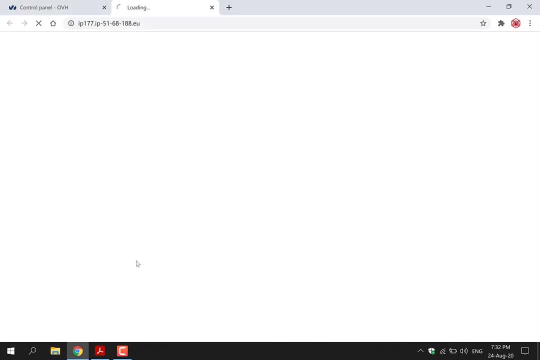 relevant to you is the WordPress application and the WordPress login URL. So let's start off with that. So all you need to do is click this link in your emails to be brought to the login page for your WordPress site, and you'll be brought to this welcome page. So let's start by entering our site name. So I'm 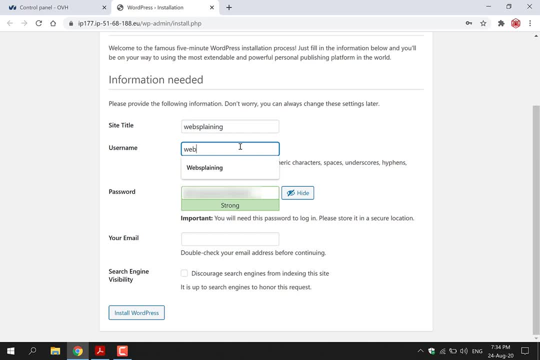 going to go with Websplaining, and for my username, let's go with Websplainer, and then for the password, Let's go with this automatically generated password For the time being. we can always change the password later on and pick an email address Once you've entered your email.